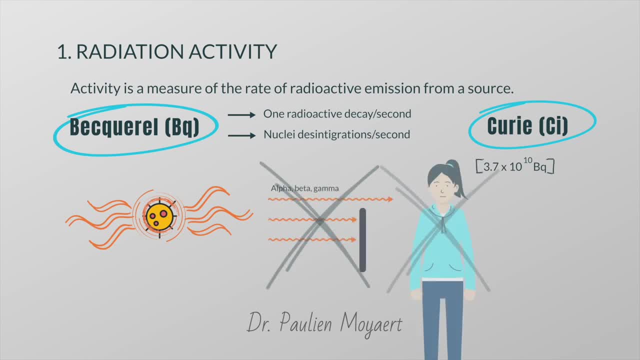 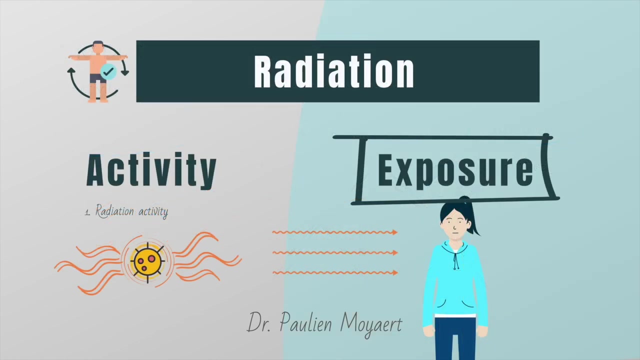 The concept of activity is independent of the type of emission, as well as independent of the material the radiation is impacting. In other words, the absorbed dose tells nothing about the radiation dose that is actually absorbed by objects. If we want to know this, then we have to look at exposure Radiation. 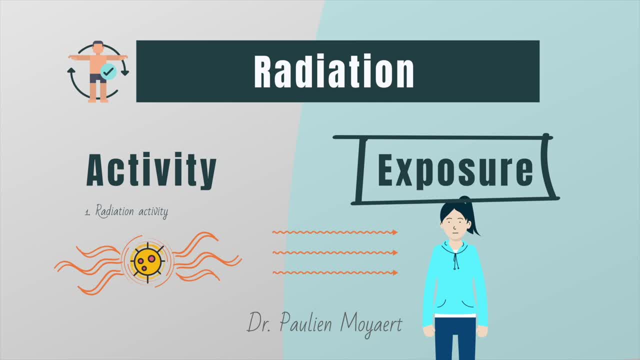 exposure is expressed in several ways. In the next couple of minutes we're going to see how radiation ends up in the error. The future of our input to the answer. we already explained this in our previous video. API outward red star problems says the question: whichstyle values? 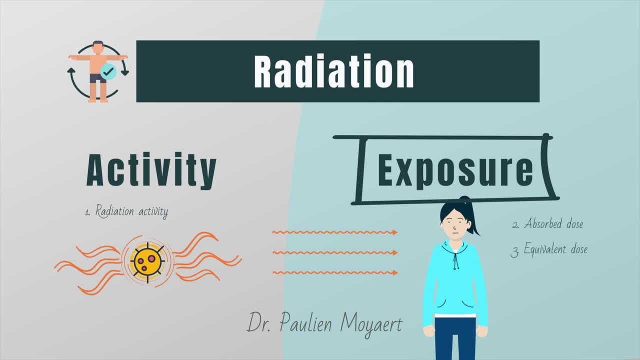 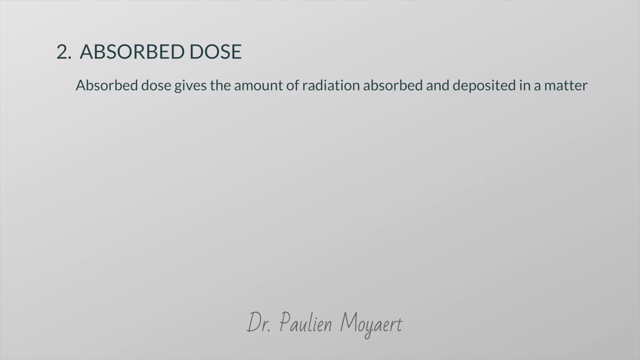 minutes. we will talk about the absorbed dose, the equivalent dose and the effective dose. The absorbed dose gives the amount of radiation absorbed in a matter, be it bone, fat, muscle or concrete, irrespective of the effects this deposit has on the material. But why do we? 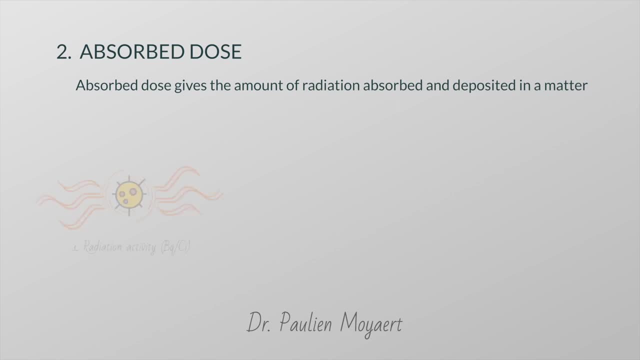 deal with the absorbed dose. We have just discussed radioactivity and the intensity of a radioactive source, But a radioactive source represents no biological risk as long as it is isolated from the environment. However, when people or another system are exposed to radiation, energy is deposited in the material and radiation dose is delivered. It is therefore 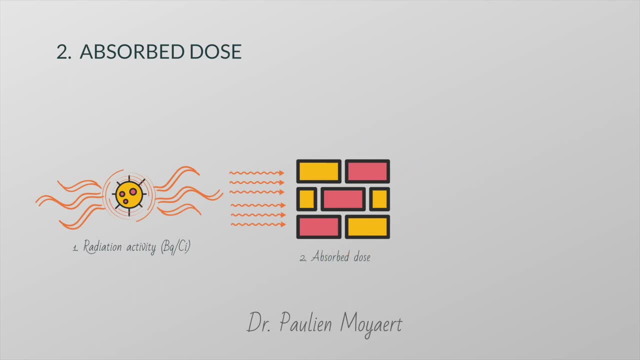 very important to distinguish between radioactivity of a radioactive source and the radiation dose which may result from the source. The international unit of absorbed dose is the QEI. This is defined as the absorption of one eula of radiation energy per kilogram of matter. 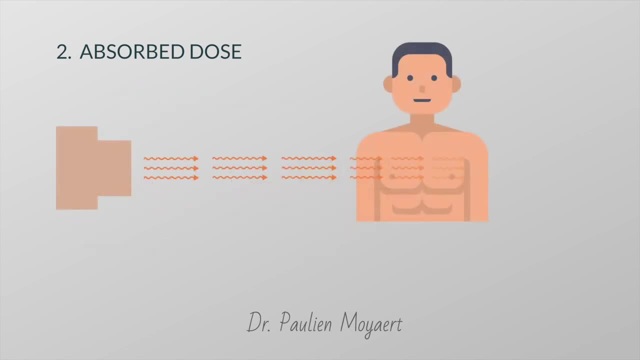 Let's give you an example. An X-ray beam will be attenuated by absorption as it passes through the body, So not all tissues within the beam will absorb the same dose. The radioactivity or the emission from the source will be the same, but the absorbed dose will be much greater. 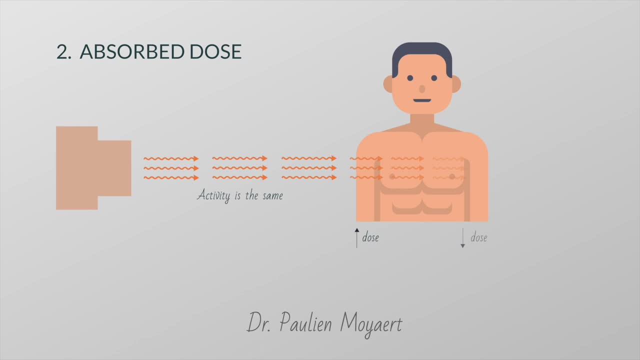 for the tissues near the entrance surface than for those deeper within the body. Another example: if you have a CT of your upper abdomen, the absorbed dose to your chest is very low because it has only been expanded by the Lucknow system to the point where the 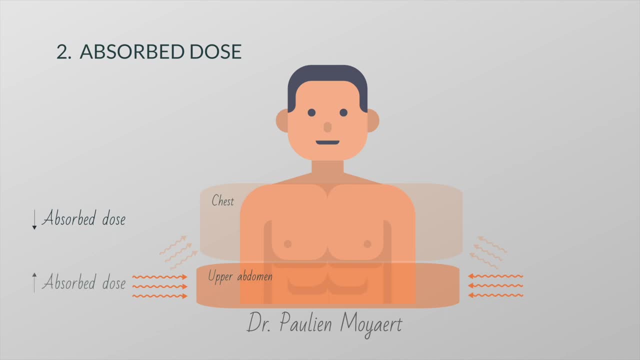 exposed to a small amount of scattered radiation. On the other hand, the absorbed dose to your stomach, pancreas, liver and other organs is the greatest because they have been directly exposed to the radiation. Absorbed dose is the amount of radiation energy absorbed in tissue. 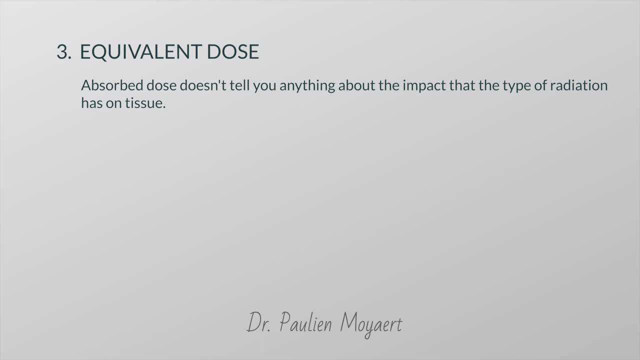 However, different types of radiation cause different levels of biological damage to tissue. Absorbed dose doesn't tell you anything about the impact that a type of radiation has on that tissue, Because, for example, one gray of alpha radiation is more harmful than one gray of beta radiation. 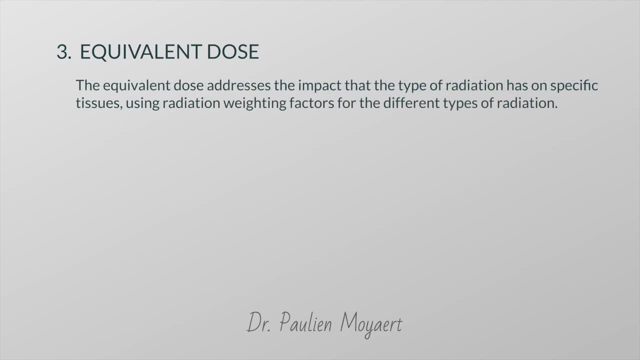 To account for this, we use the equivalent dose, which addresses the impact that a type of radiation has on that tissue. It uses radiation weighting factors for the different types of radiation. For example, gamma and X-rays have a weighting factor of 1, as do betas. 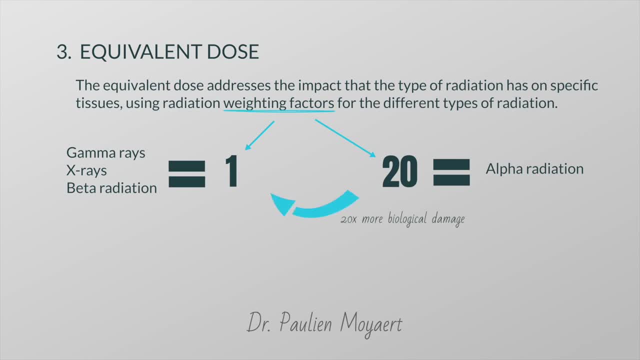 Alphas have a weighting factor of 20, meaning they cause 20 times the biological damage of gamma rays for the same absorbed dose. The equivalent dose is expressed in a measure called the sievert. An equivalent dose of one sievert of alpha radiation will have the same biological effects. 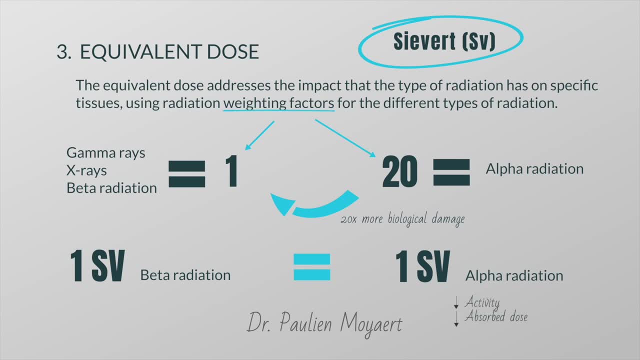 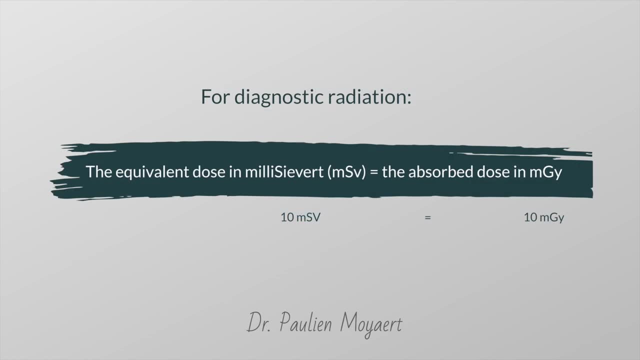 as one sievert of beta radiation, but the activity and the absorbed dose will be much lower for alpha radiation. One important note: because all radiation used in diagnostic medicine has the same low harm potential, the absorbed dose and the equivalent dose are the same. 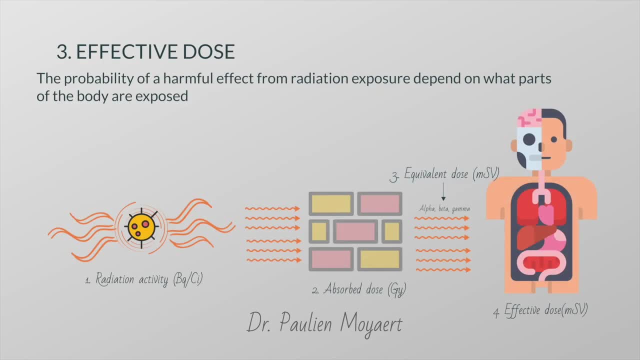 Only the units are different. 2. The probability of a harmful effect from radiation exposure depends on what part or parts of the body are exposed. Studies have shown that the risk of damage leading to cancer or serious genetic disease is greater in tissues where cells divide frequently. 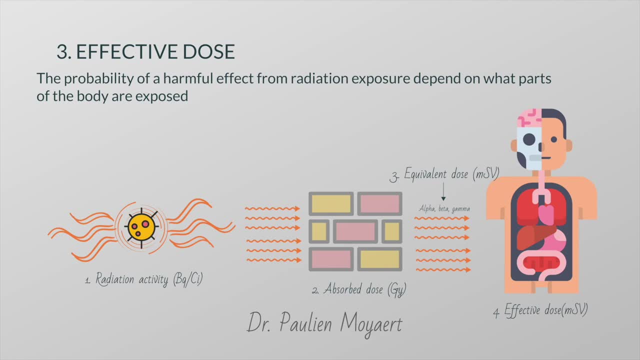 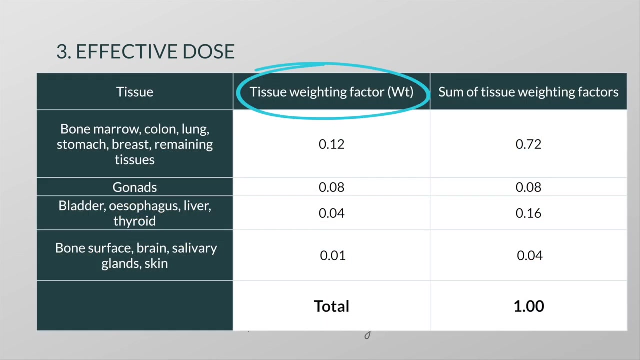 For example, bone marrow is much more radiosensitive than muscle or nerve tissue. To obtain an indication of how exposure can affect overall health, the equivalent dose is multiplied by a tissue weighting factor related to the risk for a particular tissue or organ. Here you see the different tissue weighting factors. 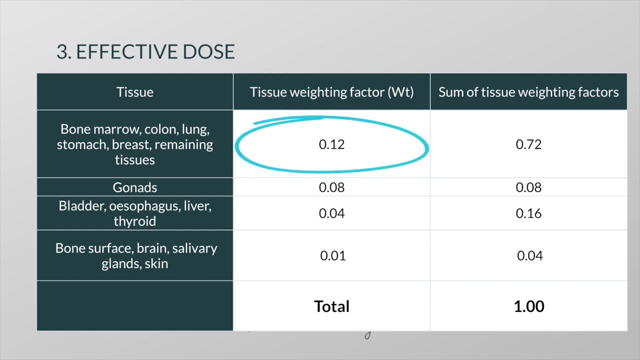 Bone marrow, colon, lungs, stomach and breasts are given a high factor of 0.12, because these are organs with a high risk of radiation-induced fatal cancer. The skin, on the other hand, is assigned a factor of 0.01.. 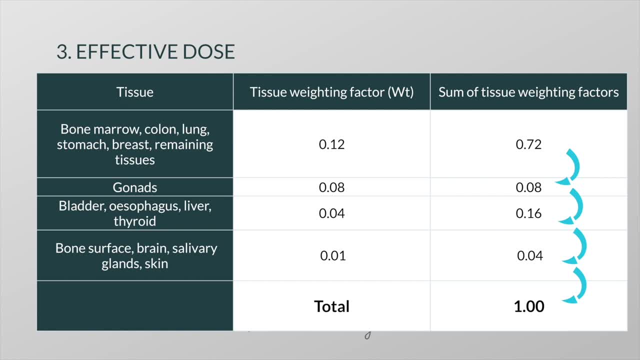 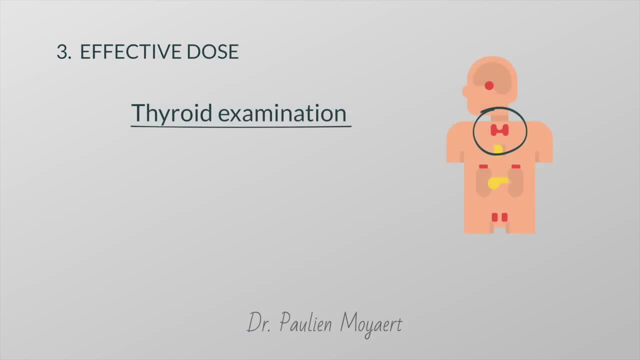 If more than one organ is exposed, then the effective dose is the sum of the effective doses to all exposed organs. Here's an example to illustrate this. Let's say it is necessary to undergo a thyroid examination. The measured absorbed dose is 10mg.